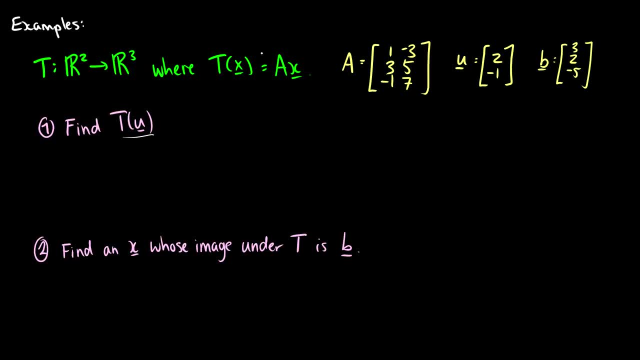 Well, this function says we take our vector x and we multiply it by the matrix A. So T of u is really just the same thing as saying A times u, And we do this all the time. We've done this a few times before. 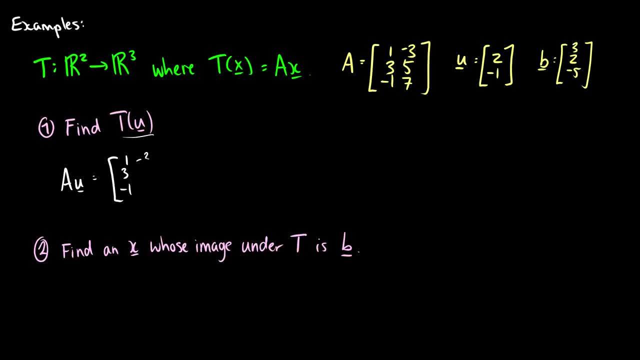 So we take 1, 3, negative 1, negative 3, 5, 7.. Then we multiply it by our vector u, which is 2, negative 1.. And we know this is just 2 times the first vector plus negative 1.. 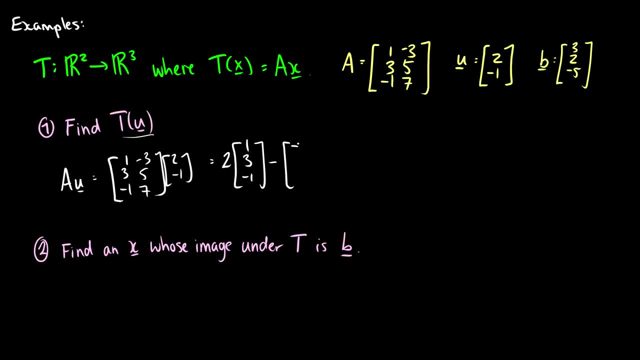 Or I should say, minus the second vector. So this is negative 3, 5,, 7.. And we get our result, which is going to be: We'll do this step by step: This is 2, 6, negative 2, minus negative 3, 5, 7.. 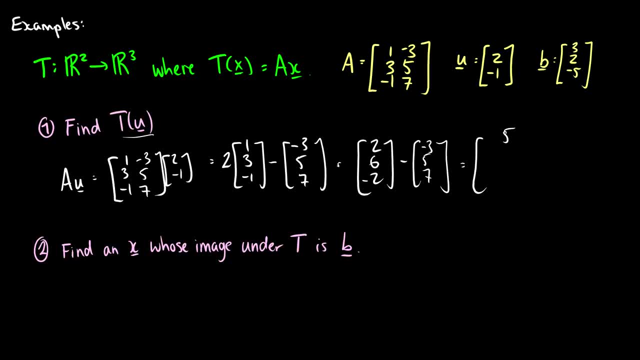 And this is just equal to 5, 1, negative 9.. So if we take our function T and apply it to the vector u, which is 2, negative 1,, we get the vector 5, 1, negative 9.. 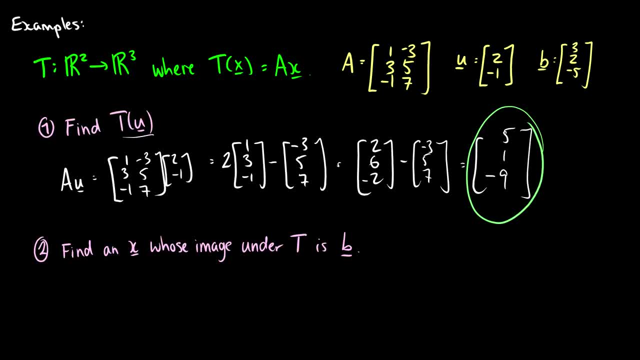 So what we can do is we can take any vector. If we were given u- and this is 2, negative 1,, we might be given a different vector, u, that's say 0, 0. And then we get a new output. 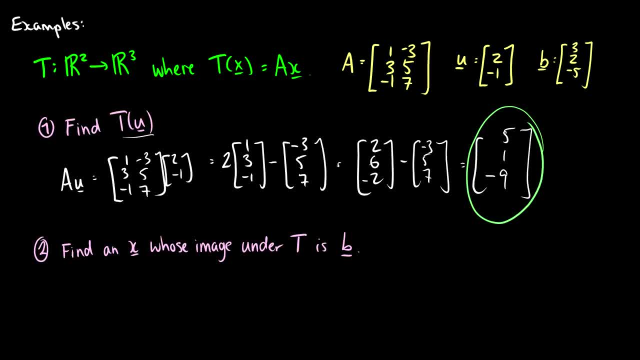 So this function takes in a vector and it spits out another vector. It takes a vector in R2 and spits out a vector in R3, which means it has two entries, And then out pops a vector with three entries. So I want to find a vector x, whose image under T is b. 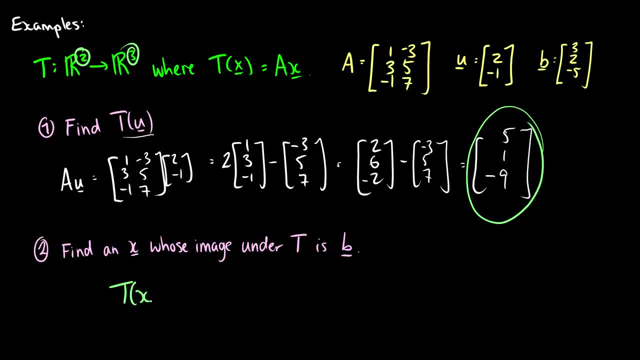 What this means is that I want to find an x such that this T of x will give us What's the vector. b, Or I should say Tx produces b. That's what I want to find. So what is b? Well, b is 3, 2, negative 5.. 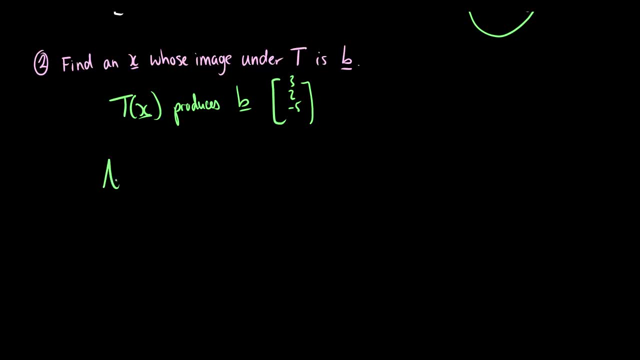 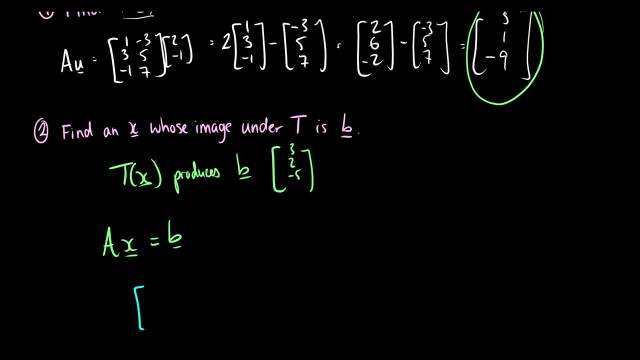 So what we're saying here is: we know our matrix A. We want to find an x such that A times x is equal to b. Of course, we've done this tons of times too. So if we remember, Our A here is 1, 3, negative 1, negative 3, 5, 7.. 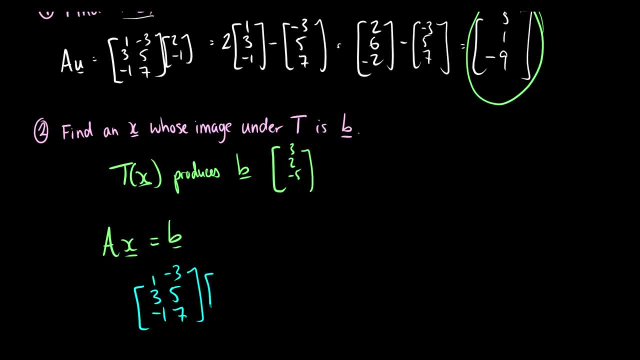 And we want to multiply this by a vector x. So of course this function takes something with two entries and spits out something with three entries. So we have x1 and x2.. And this equals 3,, 2, negative 5.. 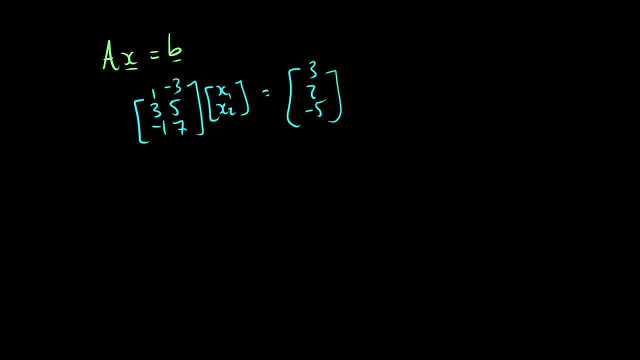 So how do we solve for this? Well, we just form an augmented matrix And then we see what comes out And we solve for our values. So negative 1, 3, 3, 3, 5, 2, negative 1, 7, negative 5.. 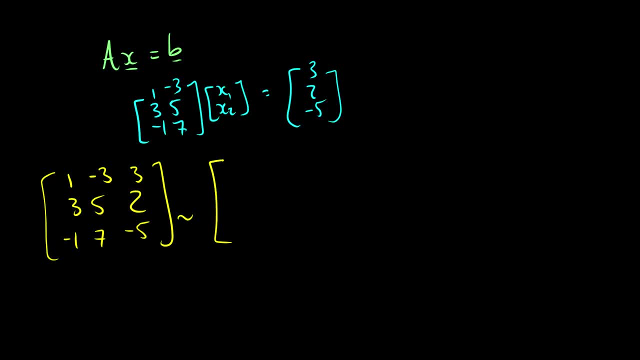 Let's see how quickly we can do this here, So the first row is going to stay the same. We're going to take the third row and subtract 3 of the first row, So we'll get 0,, 14, and negative 7.. 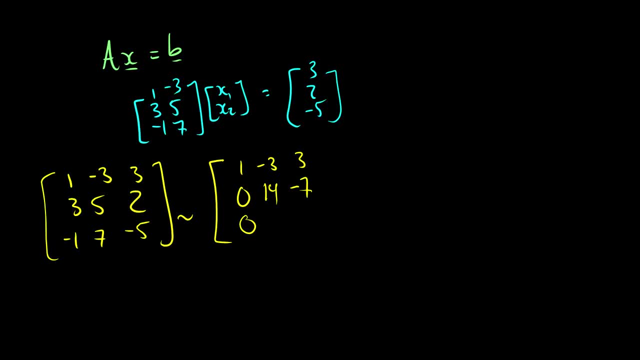 We're going to take the second row and add the first row, So we get 0,, 4, and negative 2.. We're going to divide rows 2 and 3 to make them a little bit nicer, So we have 1, negative 3, 3.. 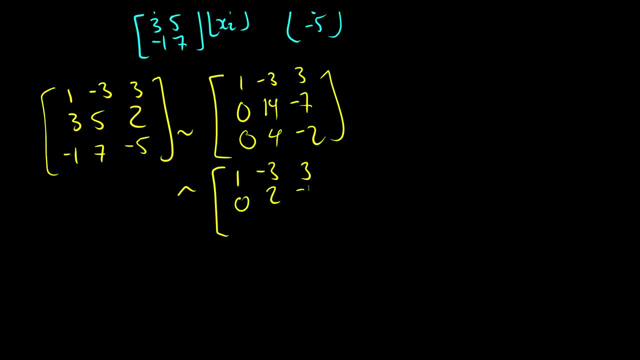 Divide the second row by 7.. So we get 0, 2, negative 1.. Divide the second row by 2.. So we get 0, 2, negative 1.. Oh, what do we see here? See, the second row and third row are the same. 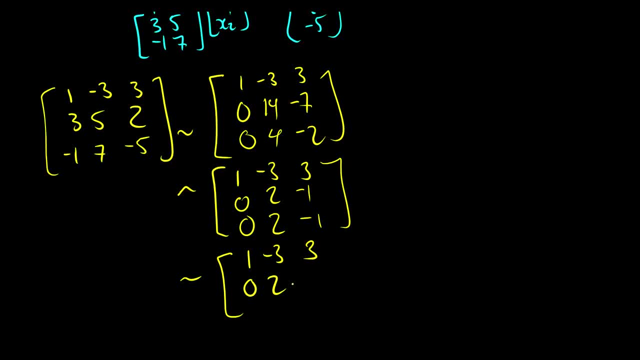 So we have a 3. We have a free variable somewhere, So this is 0, 0, 0. And now we can solve. So we know that 2x2 is equal to negative 1. So x2 is equal to negative 1 half. 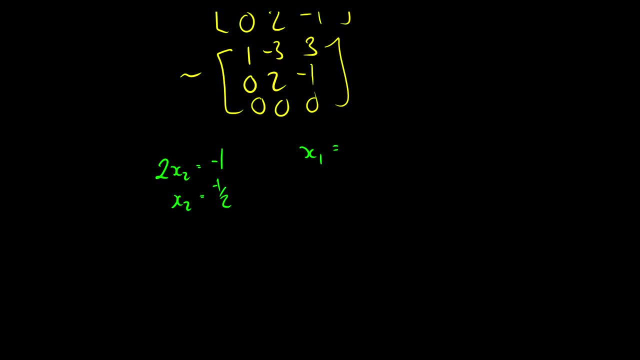 And we know that x1 is equal to 3 plus 3x2.. So x1 is going to be 3 over 2.. So the vector that produces b is x is equal to 3 halves and negative 1 half. 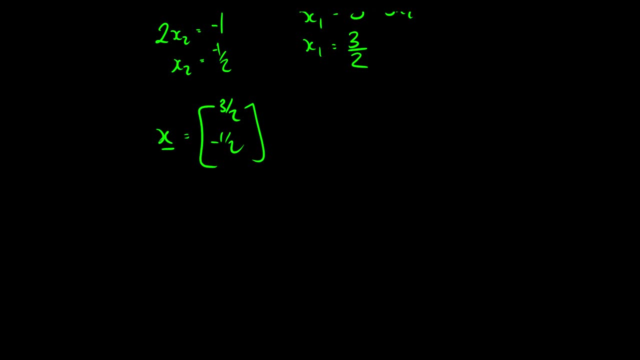 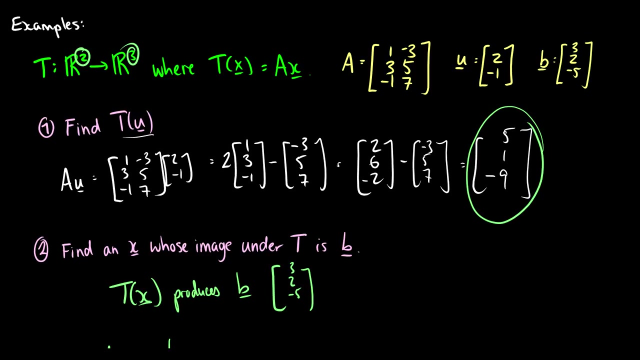 And if we put this into t, what we're saying here is that this t of this vector, 3, half negative, 1 half. this produces b, And that's the same thing as saying that ax is equal to b. So that is the point of this exercise: to find an x whose image under t is b. 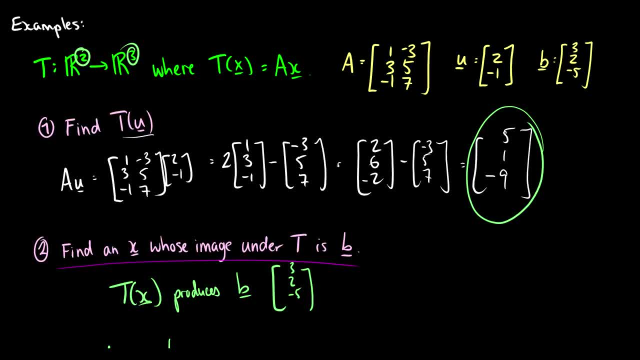 This just means what do we plug into our function t to get b out, And that happens to be a times that matrix x, which is equal to b. Then we can do some augmented matrices. We'll reduce them and solve for the vector x. 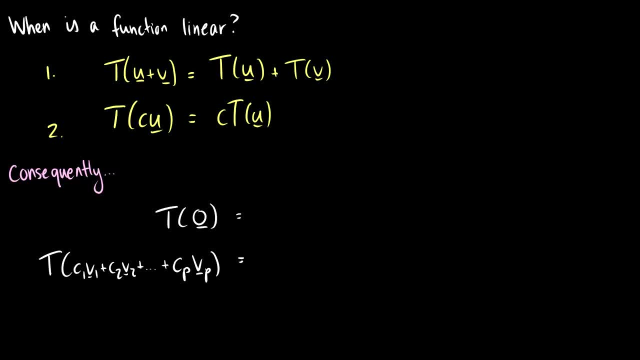 So here's a question: When is a function linear? And a function is linear? when the transformation of two added vectors, u and v, is equal to t, or the transformation of u plus the transformation of v, And when we take a transformation function and we multiply it by a scalar and a vector. 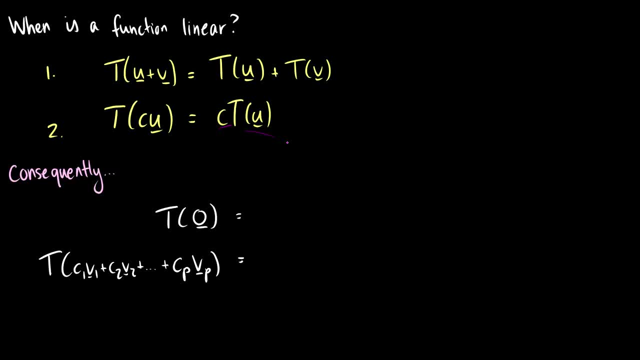 then we get the scalar multiplied by the translation. So again we can prove these. So we say that a transformation. remember. we say that t of x is really just the same thing as a times x. So what we're saying here is that this t, which is u plus v, is just equal to a times u plus v. 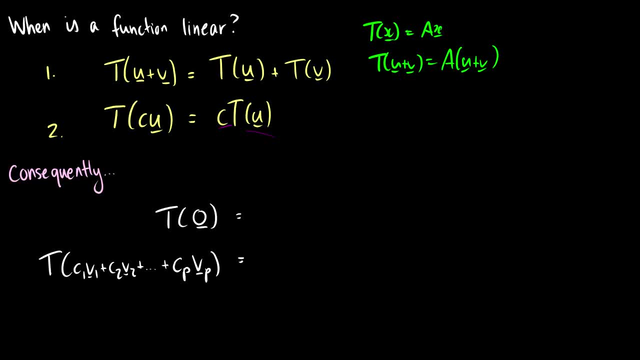 And we know from an earlier video that this is just equal to au. So what we're saying here is that this t, which is u plus v, is just equal to a times u plus a v. And what is au? Well, au is just the transformation of u and av is just the transformation of v. 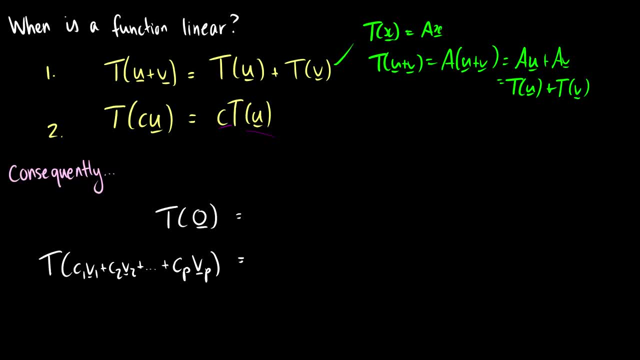 So these are equivalent And you can prove the second one for yourself using the same method. So what are the results of this? Well, this means that if we take a linear transformation on the vector 0, we get 0 back. So if we put 0 back, we get 0 back. 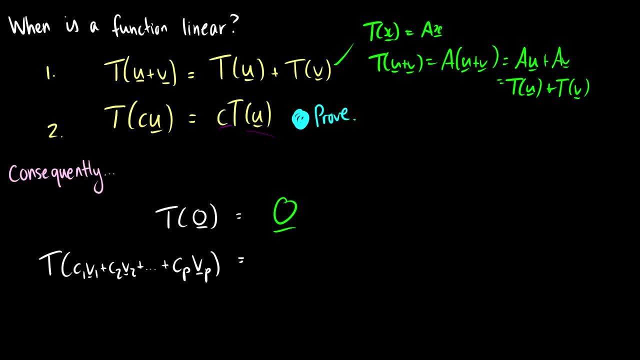 So if we put 0 into our transformation, we always get 0 back. And if we take the transformation of a linear combination, well, we just use properties 1 and 2 to get. this is the same thing as c1 times the transformation on the vector v1. 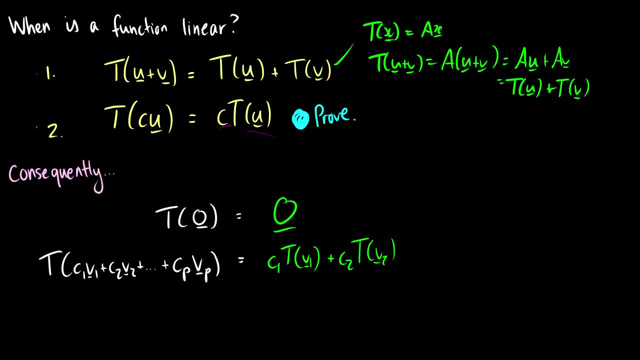 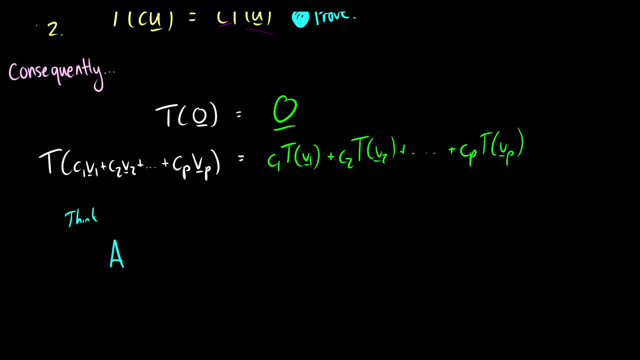 plus c2 times the transformation on v2, all the way up to cp times the transformation on vp. And if you remember, if we think about taking a matrix and multiplying c1, v1 all the way up to cp vp, well this was just equal to c1 times av1 all the way up to cp times avp. 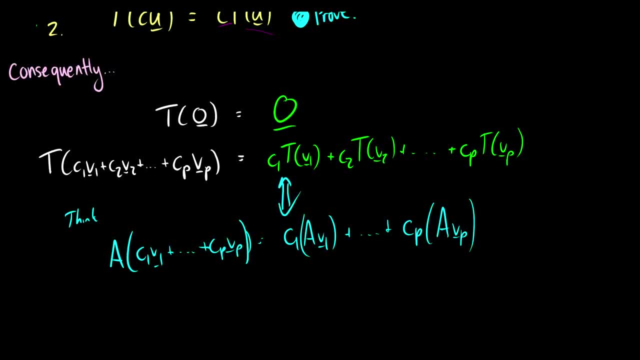 And these are exactly analogous. And again, you can prove these as well. So I challenge you to prove these ones as well, in the same method we did in the first, by realizing that this function, t, is just a matrix multiplied by a vector. So these follow pretty simply. 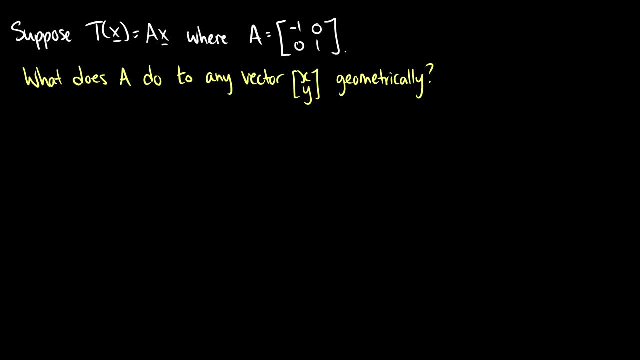 So here's what transformations are for, And in two videos we'll touch a little bit more on these. But we say, okay, suppose this transformation on x is matrix times x, where a is this matrix negative: 1, 0, 0, 1.. 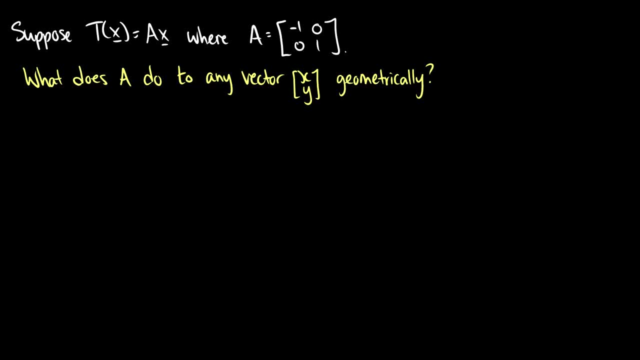 What does a do to this vector x- y? So let's plug tx in. So we're going to plug t of x y into our equation. So this is just negative 1, 0, 0, 1 times the vector x y. 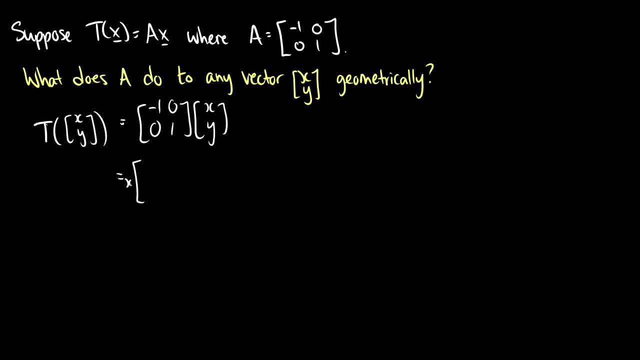 And what did we get out of this? Well, this is x Times negative 1, 0. Plus y Times 0, 1. Which is just negative x 0. Plus 0, y, Which gets our result: negative x- y. 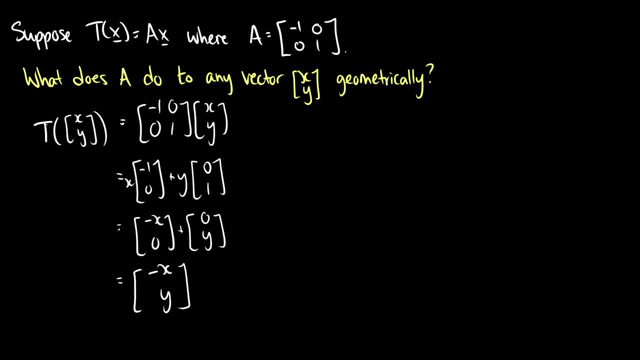 So this transformation takes a vector x- y and spits out negative x y. So we can say: okay, this takes x y And it maps It to negative x y. So suppose I have a vector that is say, let's say this is 1, 2..